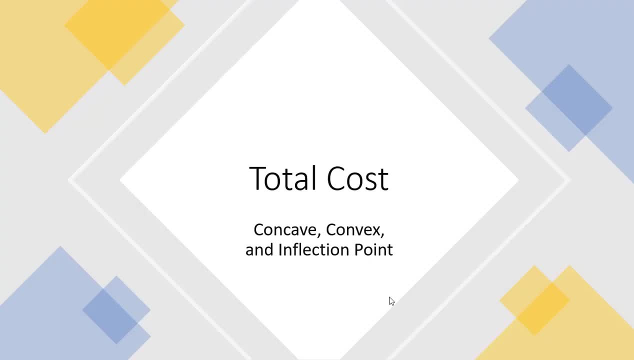 Hello, in this video we're going to determine whether a total cost function is concave at a certain point or convex at a certain point, And also we're going to try to find the inflection point on the total cost curve. Here is our cost function, where q is the quantity of output. 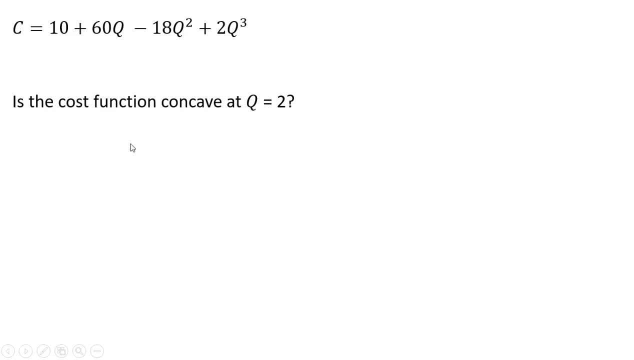 Is the cost function concave at q equals 2?? If the second derivative of the cost function is negative at q equals 2, the cost function is concave at that point. And what does that mean? It means the tangent line on the cost curve at q equals 2 will lie completely above the graph of the function, above the cost function at or near q equals 2.. 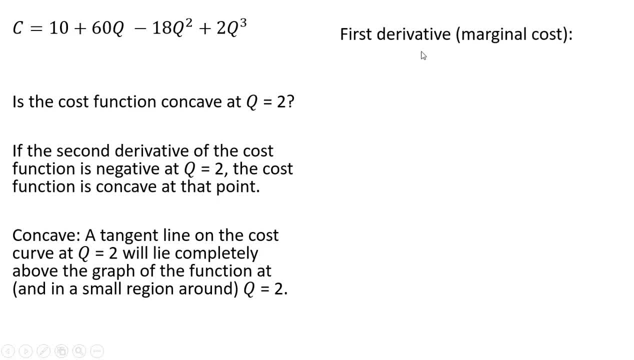 So we need to get the second derivative. So the first thing we do is get the function, We get the first derivative, which happens to be marginal cost. So taking the derivative of this equation, the derivative of 10 here, that's just going to drop out at 0.. 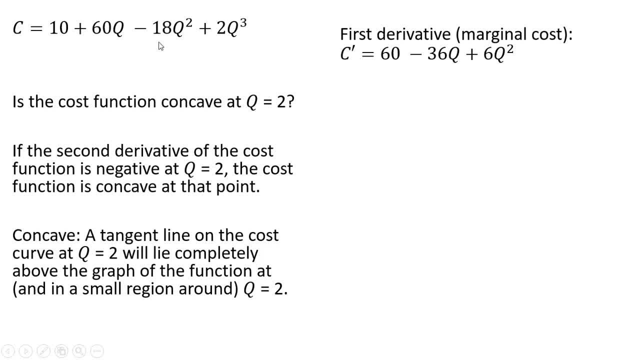 Derivative of 60q is 60, the derivative of minus 18q squared. bring the 2 down in front, so 2 times 18 is where the 36 is coming from, And then we're going to subtract 1 from the exponent here, so we're just left with q and then likewise the derivative of this final term. 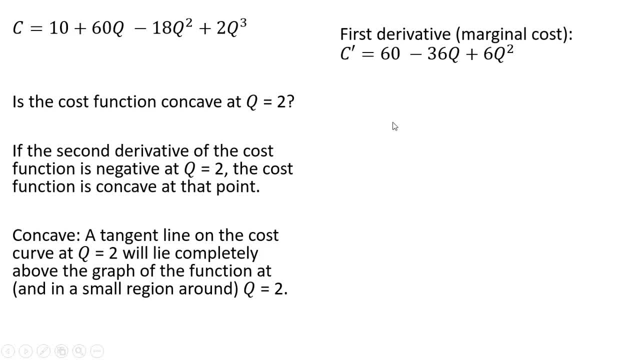 is going to be 6q squared. Taking the derivative of the derivative or the second derivative, we get minus 36 plus 12q. We're going to evaluate that second derivative at q equals 2.. And, as you can see here, the second derivative is negative. 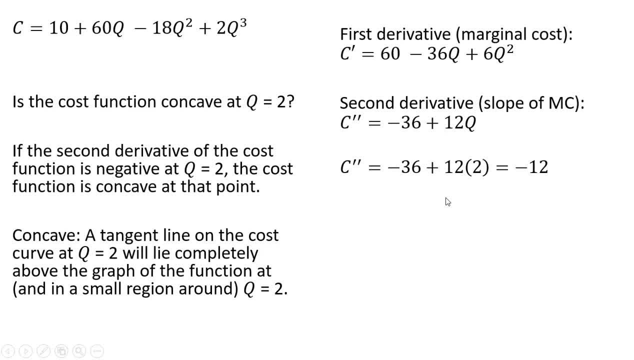 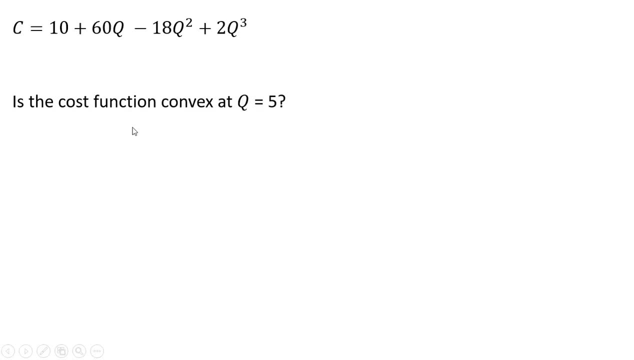 Minus 36 plus 24 equals minus 12.. So where q equals 2,, the graph of the cost function is concave. We'll look at the actual graph in a minute here, Moving on Taking the same cost function, but this time looking at whether the graph of the cost function is convex. at q equals 5,- a different point. 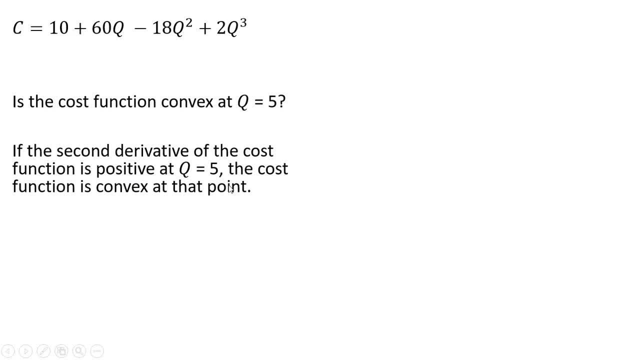 Here. if the second derivative of the cost function is positive at q equals 5, the cost function is convex at that point. What is that? What does that mean? A tangent line on the cost curve at q equals 5 will lie completely below the graph of the cost function at or near q equals 5..